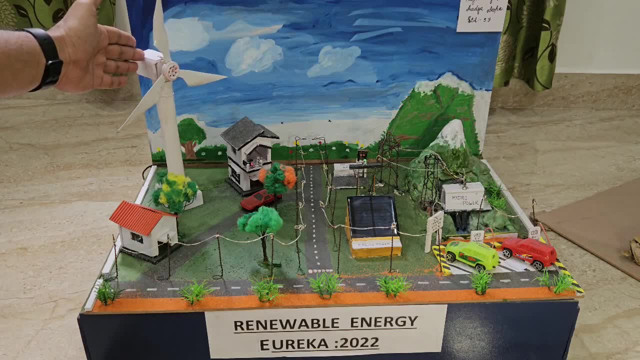 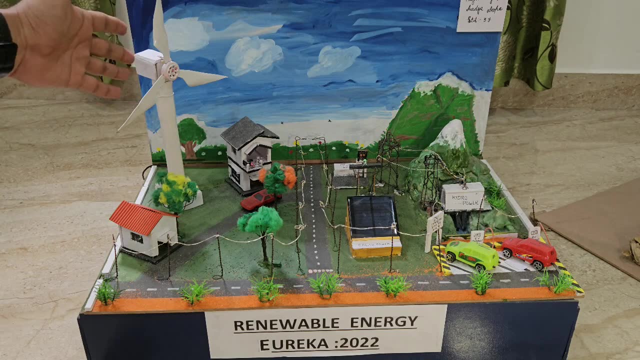 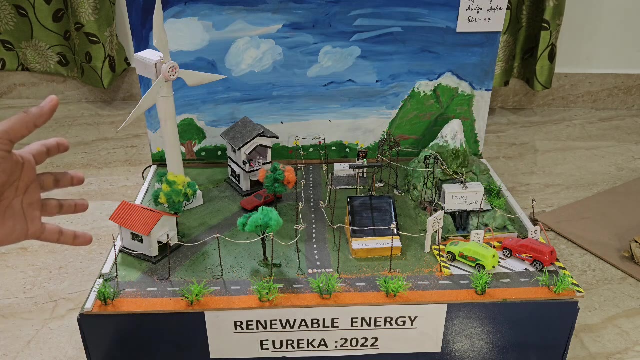 there's a wind fans over here and a wind turbine behind it. It's all working, So it's all powered by the batteries that you can easily found- that can be found on Amazon, You can order it online- and materials, all the materials that are being used in this project. 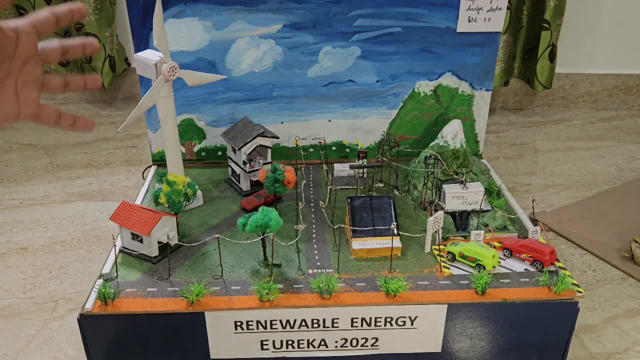 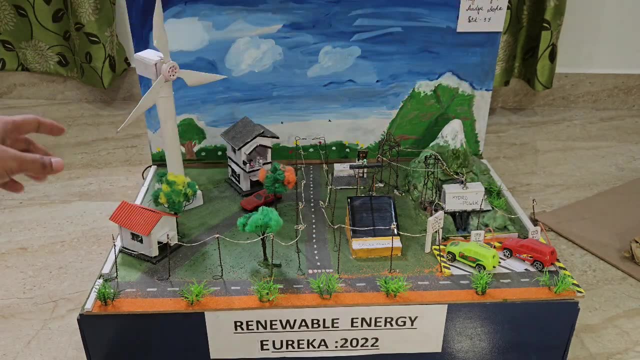 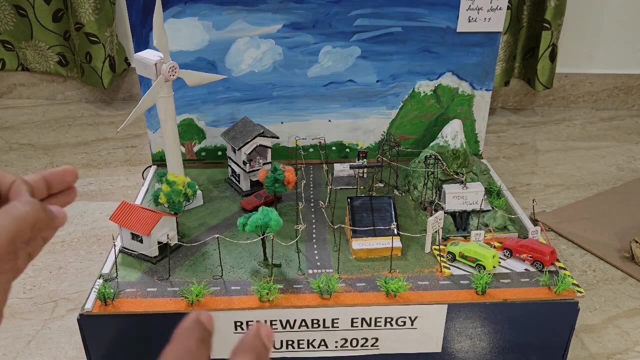 They are all homemade and they're built from scratch up, So let's discuss. So the second one is the solar power and the third one is the hydro power. Everything here, you see, is working, So let's discuss. I'll just go on to share the measurements and how it was cut, the material used. 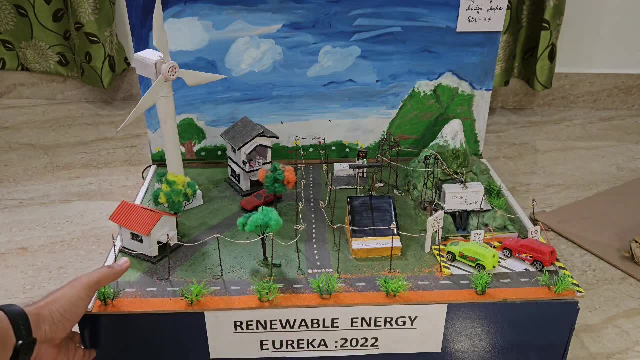 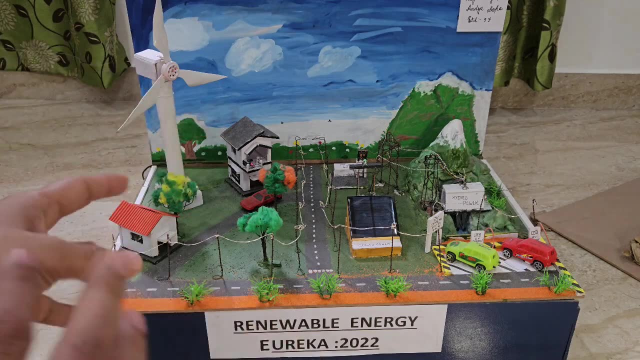 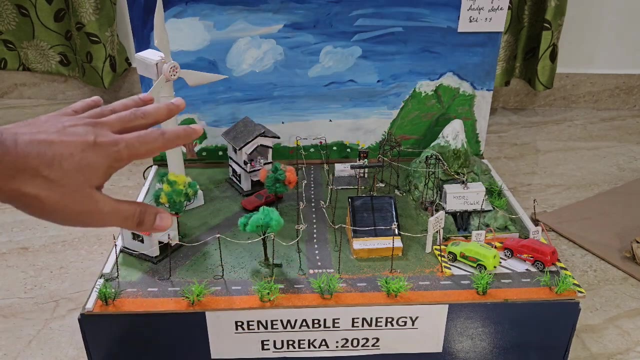 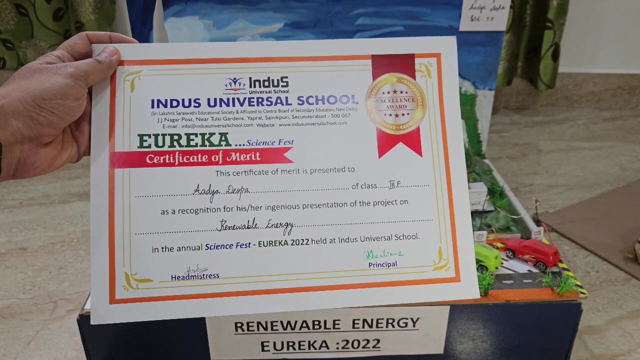 and each and every detail. And underneath this hood, underneath this box that you see over here, is all the connections that would be batteries. You can just use batteries according to your convenience. So let's discuss about this project. This was well recognized by the school and she was provided with a certificate of merit for the 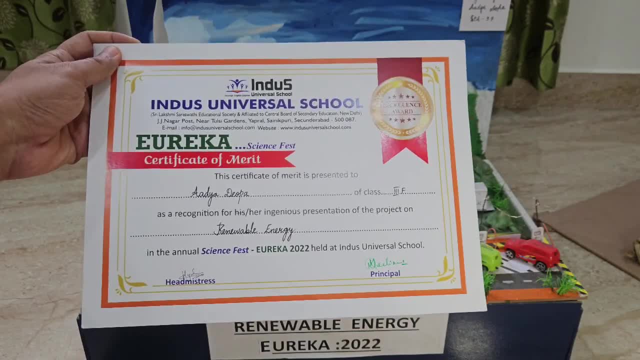 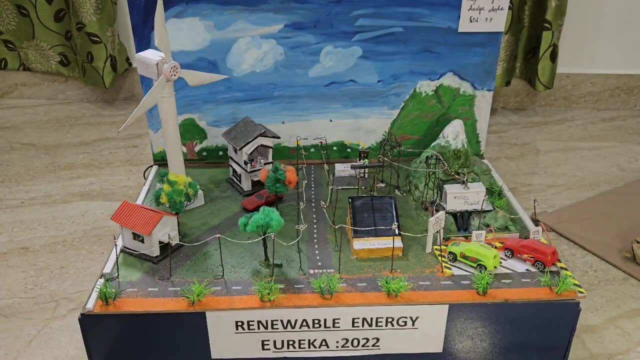 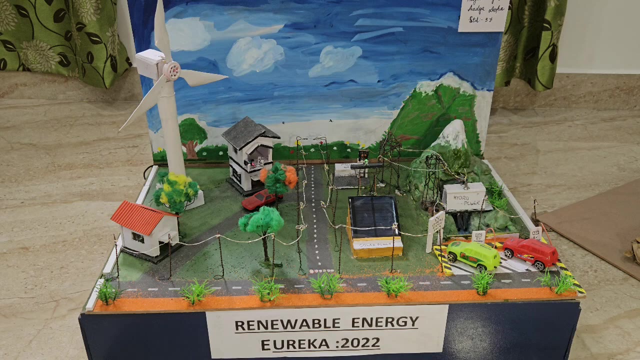 this wonderful renewable project. I was so happy that it was recognized and the effort was well recognized. So let's dive into the details. First, this board. This is a board that is ordered online. I'll just show you how big these boards are. These boards are: 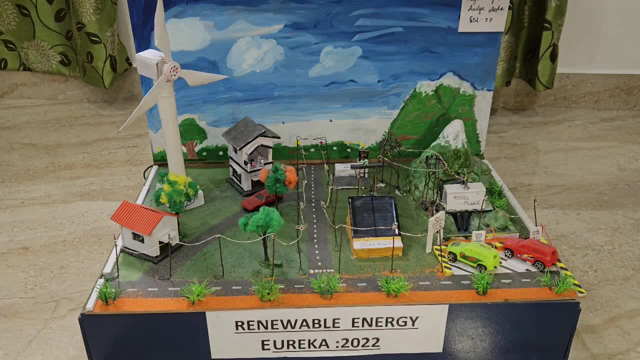 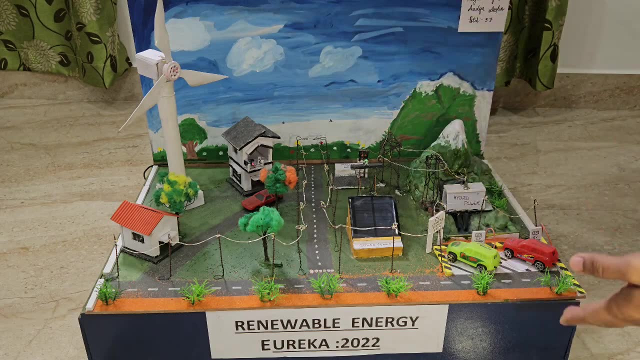 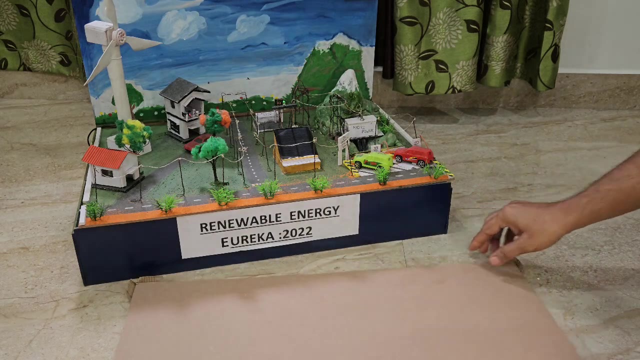 exactly the size of what I have used. This is one of the board. It comes in these sheets. This is hardboard that you can find in Amazon, So I have cut two various sizes. I'll just measure the size of this board for you to better understand how this works. So here's the measuring tape. So it's around two feet 61 centimeters, So it's a standard size that you get in Amazon, two feet in length and it's a 41 centimeters, a little more than one feet and around four inches. So this was the measurement and hope you can see It is two feet and one feet and four inches, So I have used a basic conforming. 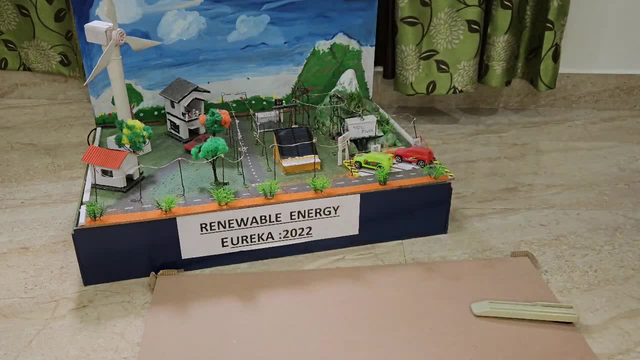 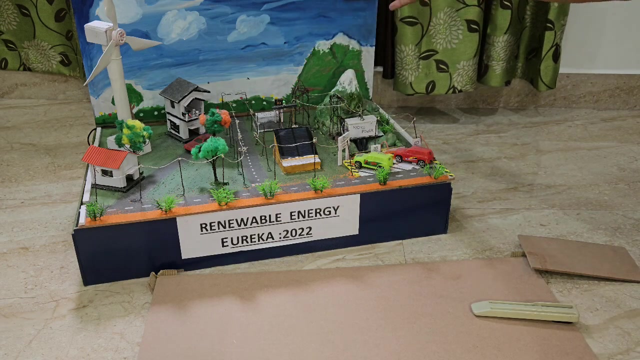 Basic cutter. This was the cutter I used to cut it into pieces, small pieces for this part, And around 5 or 6 sheets were used in whole together. This is the full sheet over here and this is one full sheet And this is the acrylic color. You can use whatever color you like to have. 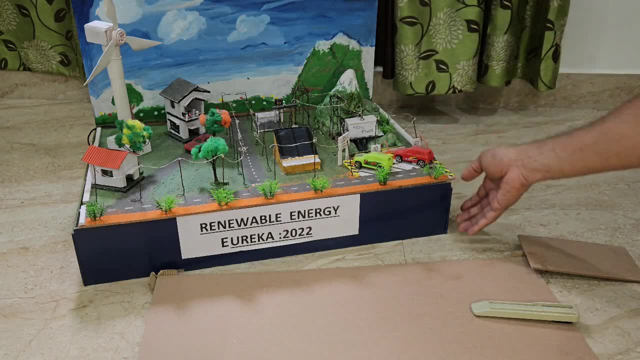 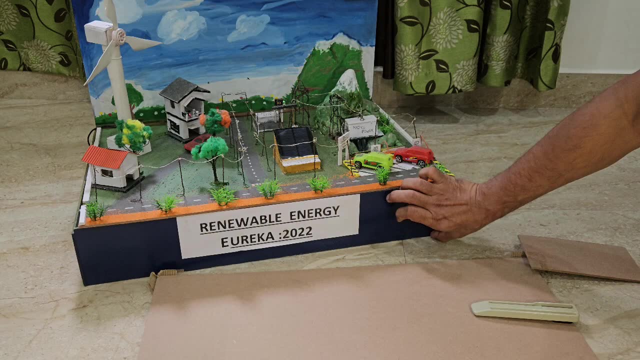 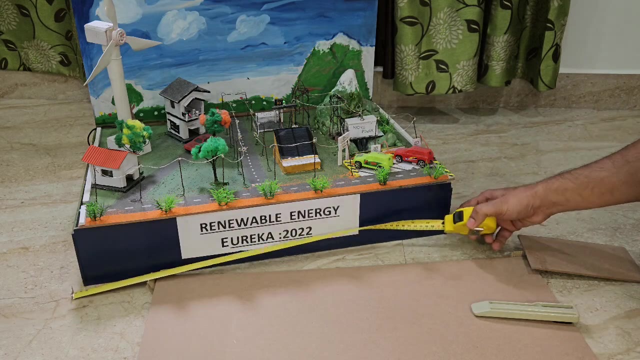 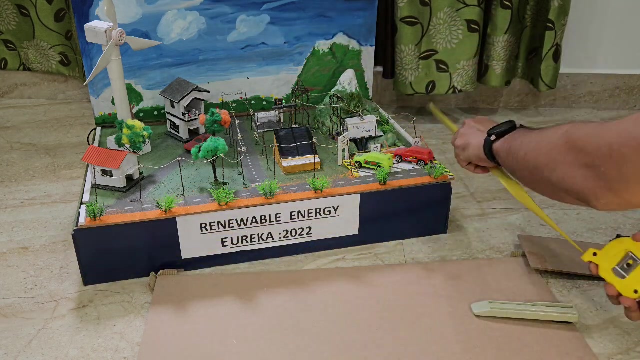 So this is one full sheet and the second full sheet and the third one is the under sheet that was used to build. These were the three sheets and few of the sheets were cut into these pieces just to measure. So the front sheet and the back sheet were of the same size, So it was around the same. It was just repeat. From the sides it was the same, It was around. I cut it in half. 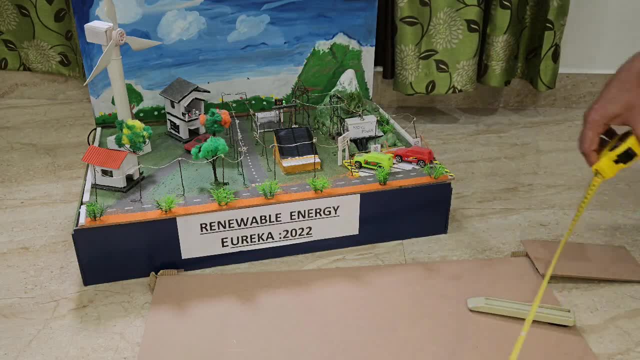 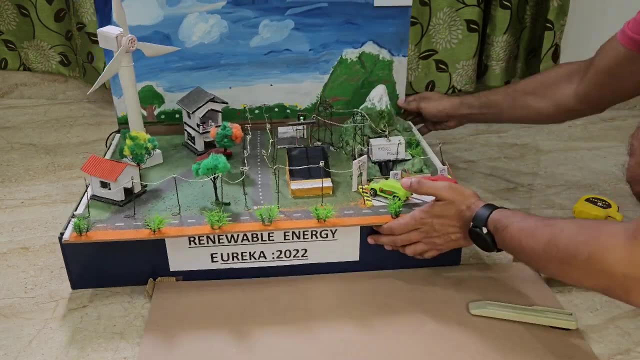 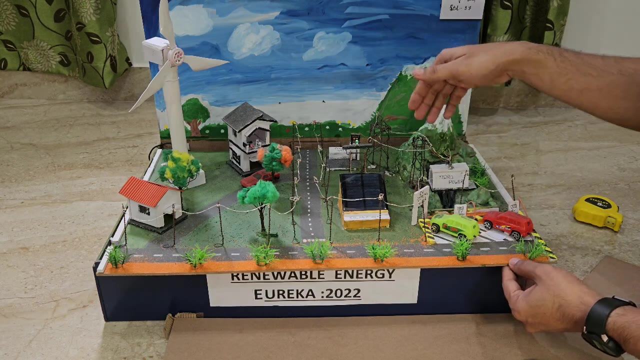 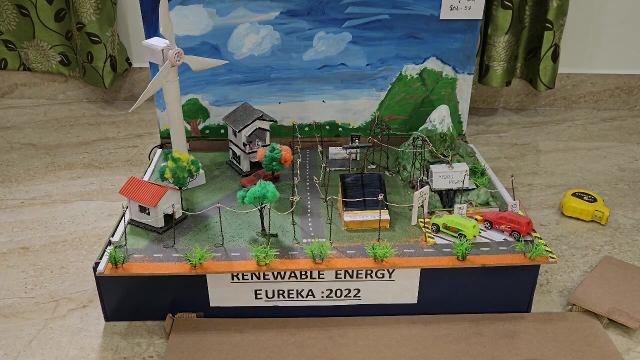 And I cut it into one piece Up to this length. Up to this length it was done. So let's test this. So, coming over to this project again, So the upper part, it was all painted first. So what we have here is the string light that you will find. I just turn it over So you can easily see. So what I did is I fixed the string light. 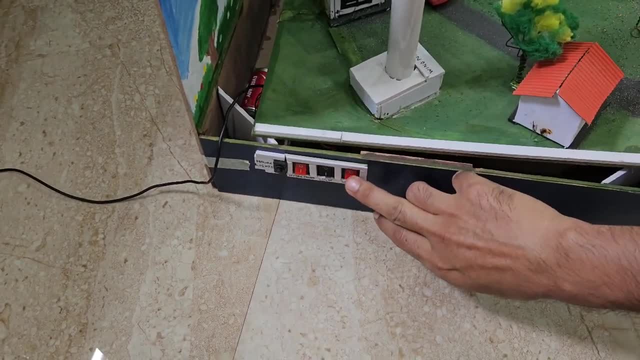 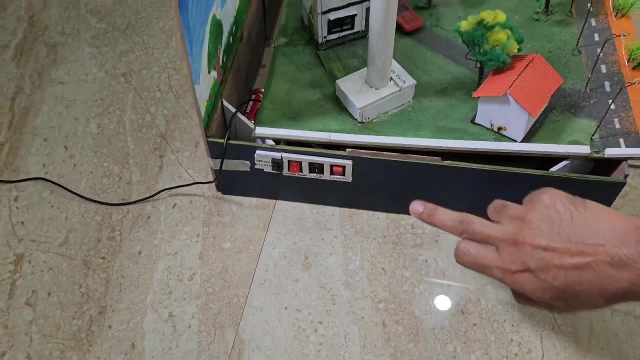 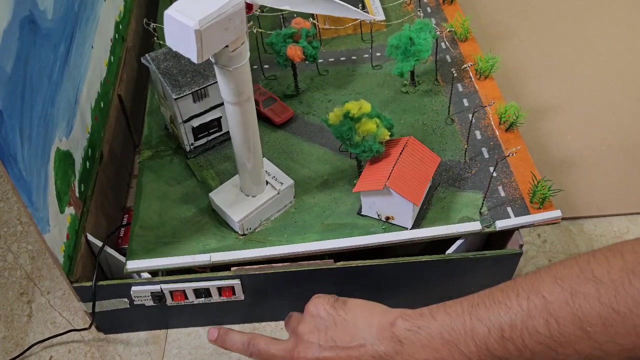 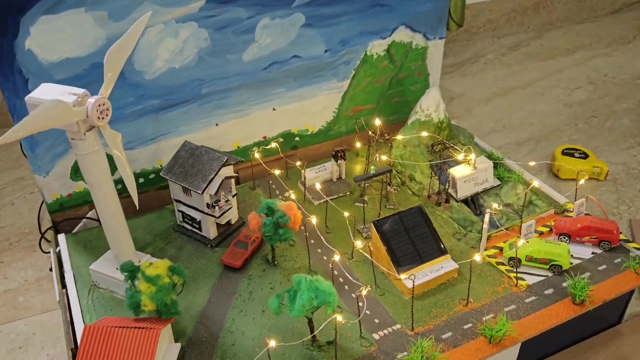 Some of the switches that I found ordered online on Amazon, So these are all connected through the connections. So when you turn it on, this ring will go off. Here it is Makes little noise, So I am turning it off. Okay, here it is. So second one was the light. So these were the string lights that was connected through the connection to the switch, So I will just let you know how it works. 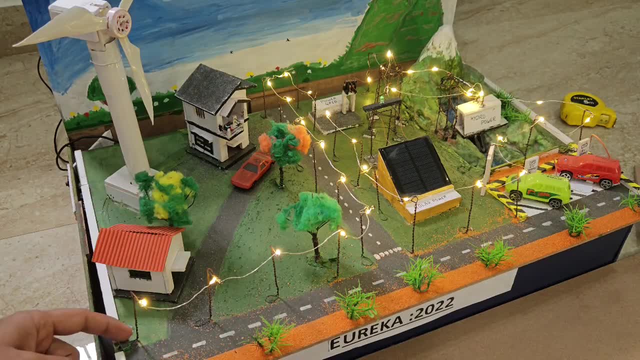 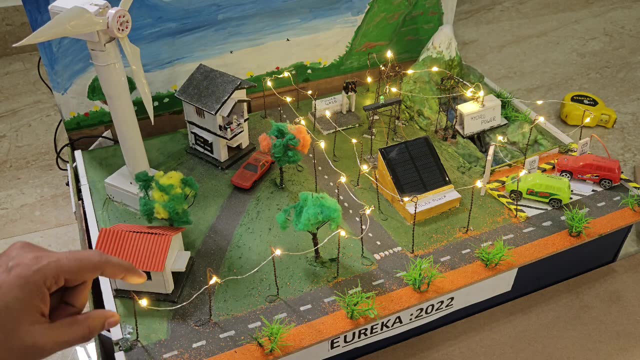 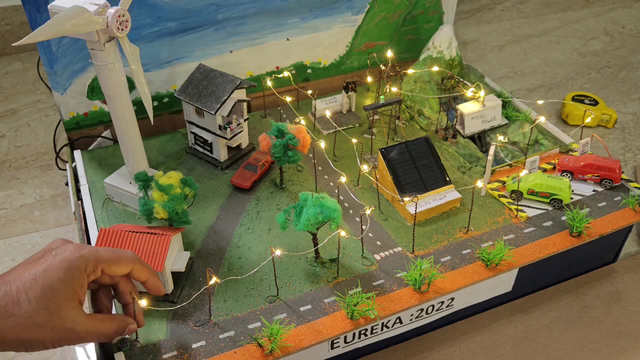 So it was all connected. So these are the string lights. Now coming over to these poles: Electricity poles that were made out of the wire that you will find in the hardware store where you find paint and everything. There you will find these wires. These are basically soft iron wires. You can cut it through the plier, So I just twisted it over twice and turn it to look like a pole, And these all were pasted. 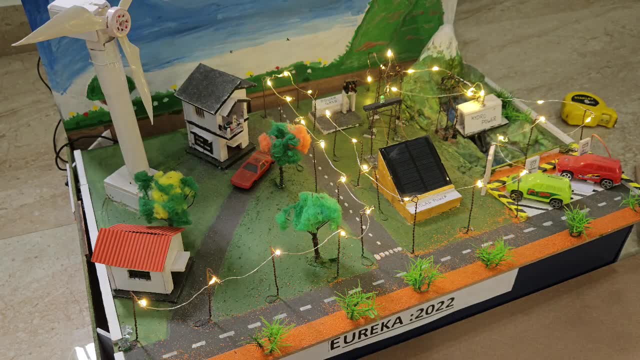 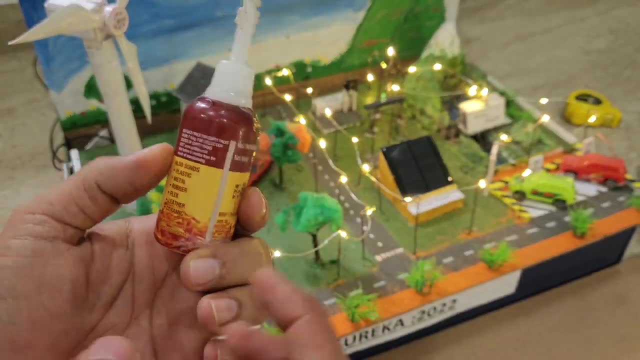 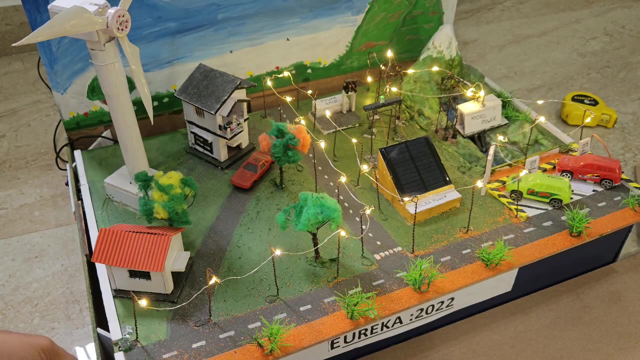 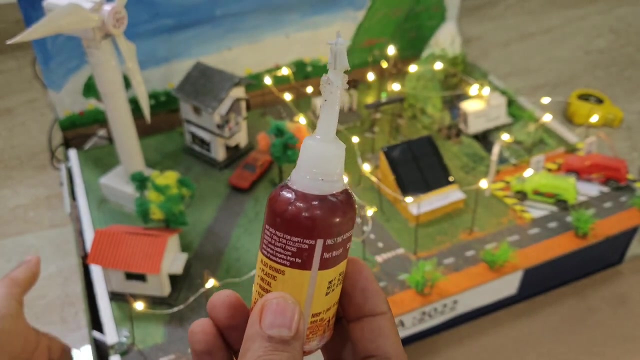 These are everything. These cut pieces and everything were pasted within fabric glue. Here is the glue that was used to paste. This is, in fabric, called brand glue. You can use any brand, but it has to be like a quick fix So it sticks very easily to this board. You just have to place these two boards together and just put. It's a very thin glue. You just put it over and it sticks quite hard to it. So what I did? I just first made this box, that is. 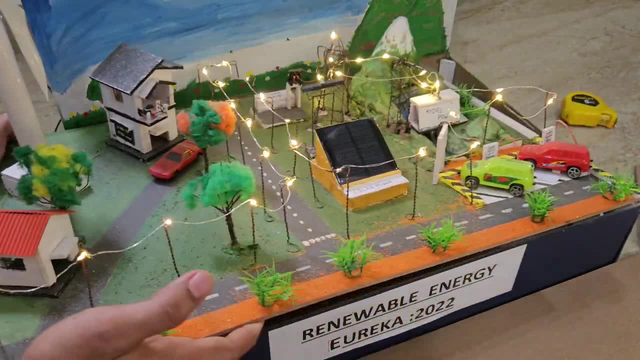 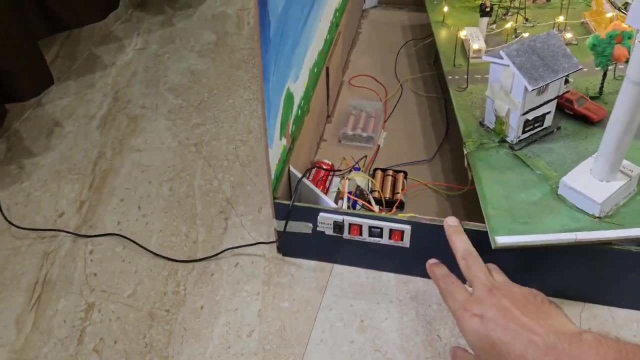 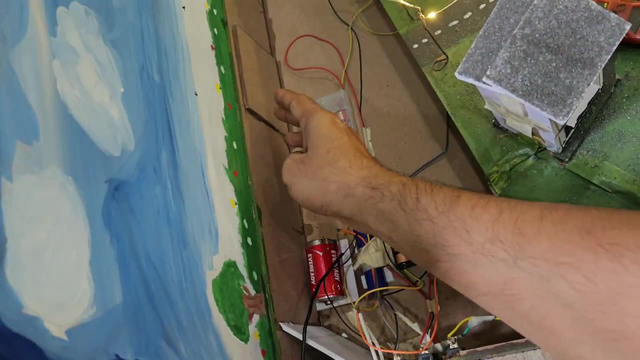 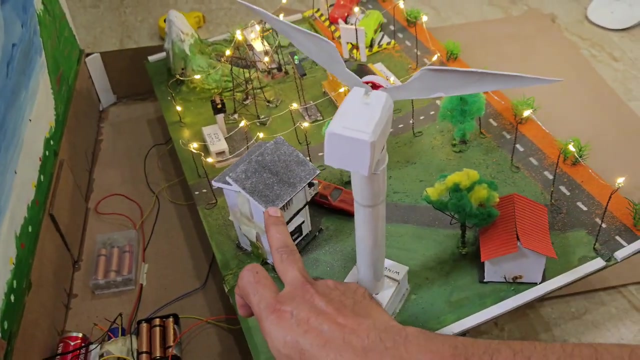 under here. So it was built. I will just show it to you. So it's a box that was built first. So you had to build this box by cutting the pieces of this length And what I did, I provided additional support to this board by this and these sheets. I put it here. So, talking about these houses that were built, That were built not from this hard board, That were built from this hard board, 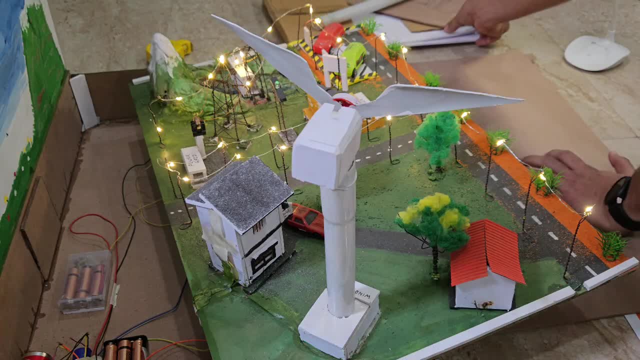 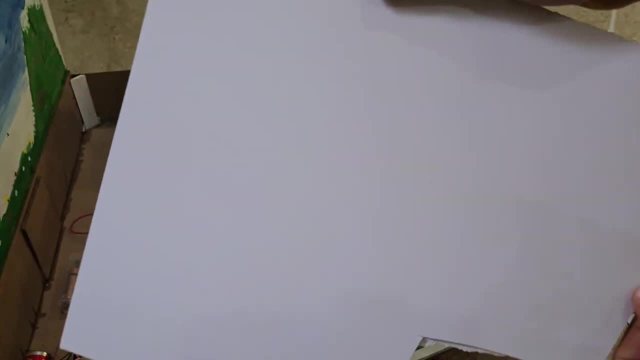 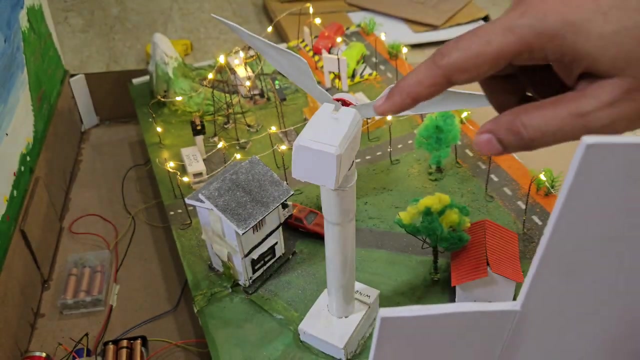 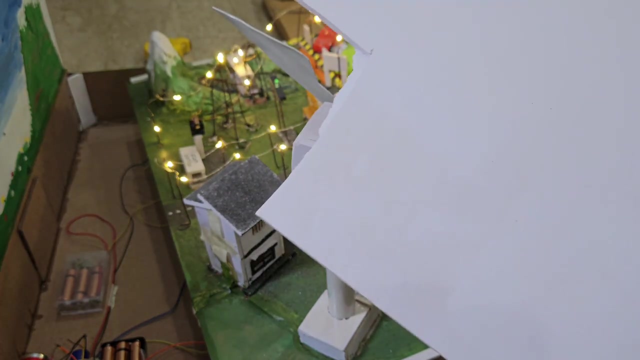 That were built from this modeling sheets that we have. These modeling sheets- or you can see, these are the foam sheets that are bought from Amazon. These also come into various sizes, So they are not needed much in bigger in size because we had to cut them into small pieces. Even this back of this windmill was built out of it. So here is this modeling sheet that also you can find on Amazon. You can order it online, So you will get it there. 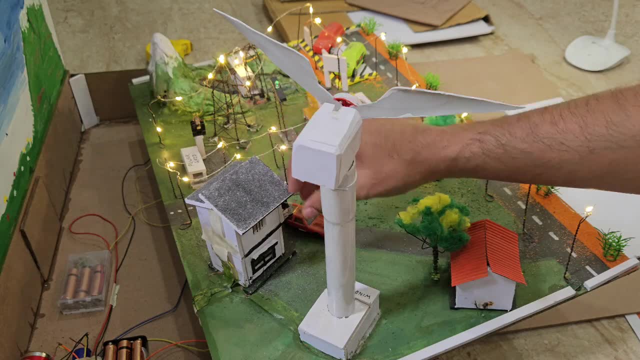 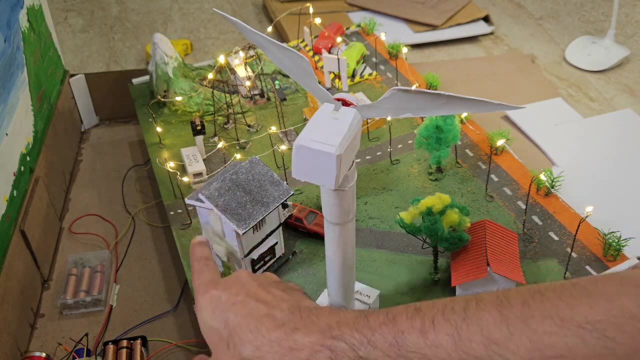 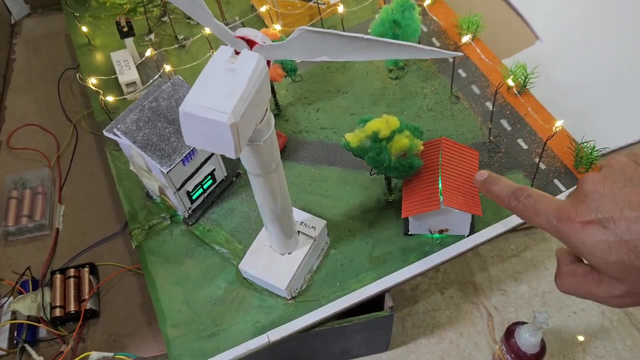 Talking over to these houses. I just cut it for the roof. Small pieces, Even the windows and these parts were cut. So before putting the roof, I just put it some LEDs. That was also ordered online So that was connected to a battery and connected with a switch over here And I press it. These lights glow inside the houses And they really look wonderful. This is a very amazing project. 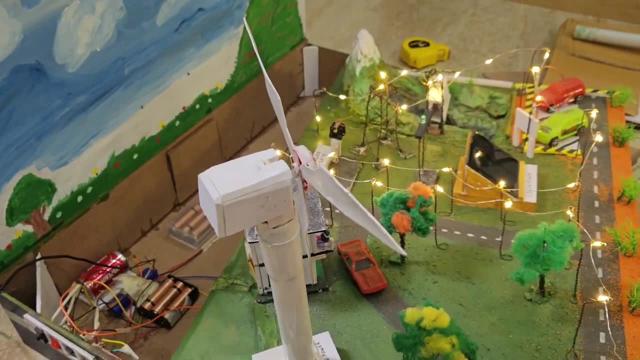 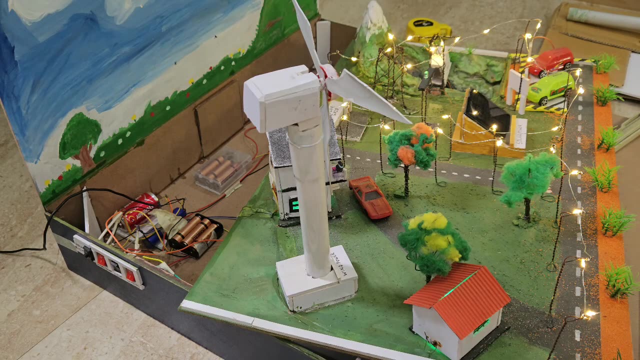 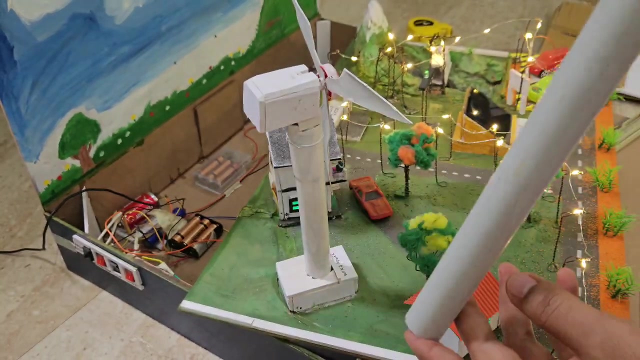 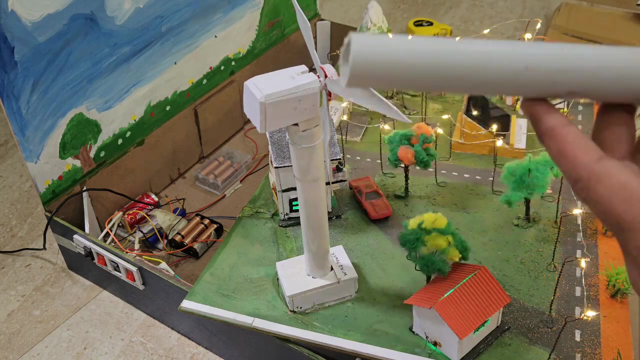 Coming over to the windmill, How it was built. So for the windmill, What I did? I used a PVC pipe, Electrical pipe. You can find it in any electrical store. So this kind of electrical PVC pipe I used. I just cut it And just poke a hole inside this upper sheet of the board And just placed it like this. And what also I did to build this shape of this windmill. 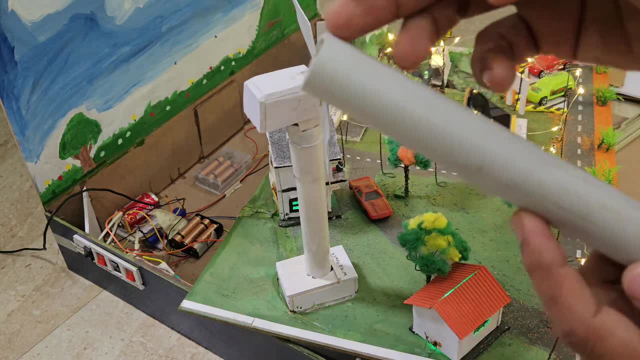 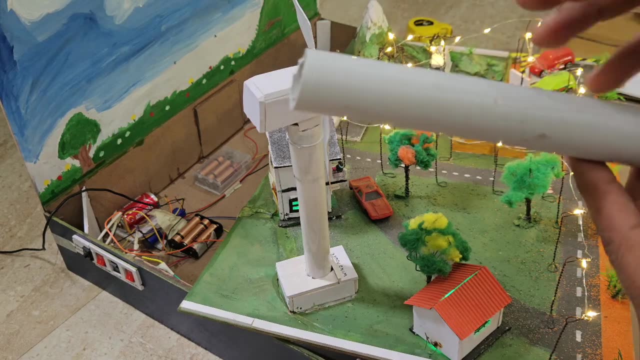 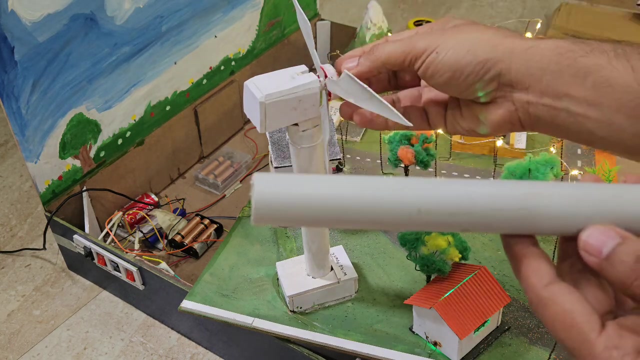 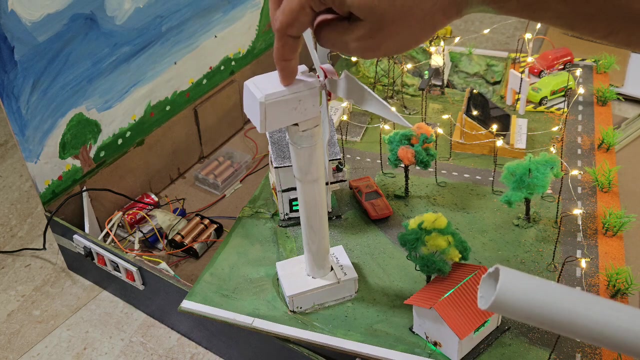 I used these blades. I just cut it through here, Heated it And just cutted it. You can just heat it over the gas or some stove or any other to heat it up. So when you heat this pipe it melts and it bends the shape and form you want to make. So I cut it over here. I used an old toy car wheel to make the center of this And I just pasted it over here. Under this there is a motor that you can find in Amazon also to make the robotics and everything that you can use. 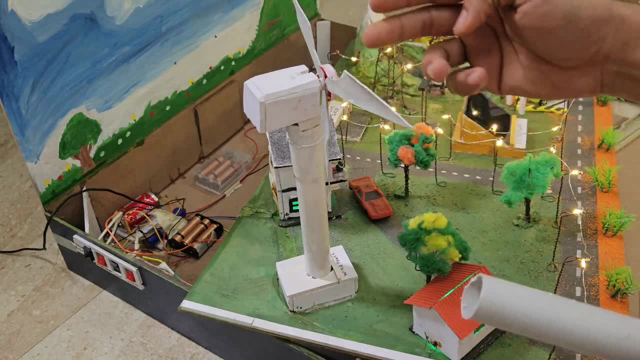 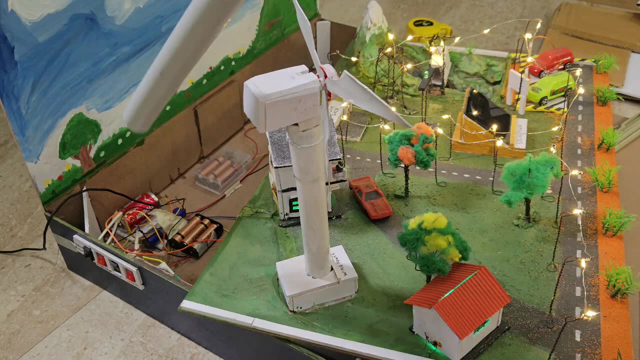 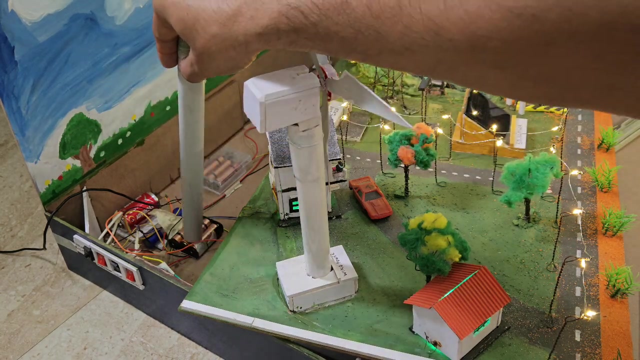 of a. it has a. it is a gear motor so the speed or the rotation speed matches with the battery so it doesn't rotate too fast when you use it with the battery. so batteries used are simple double a batteries. with that you'll find this battery pack or this to hold the batteries. 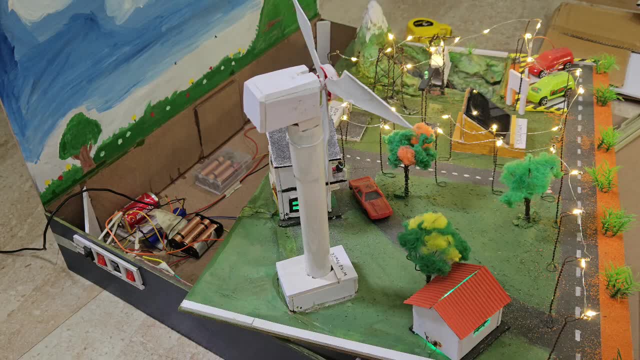 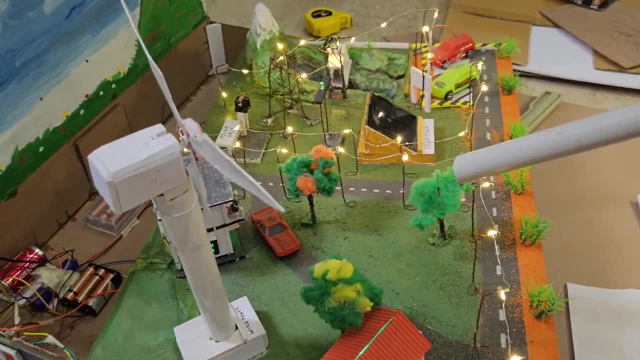 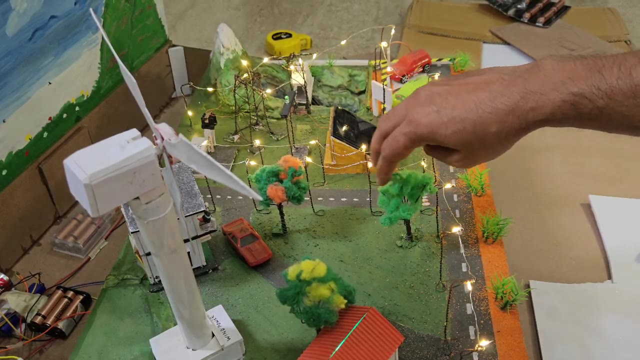 and that comes with the standard as the part of things you'll order. you'll find everything online, okay. so next, uh, coming over to these trees that i built to use again the same wires. and this is just a cotton. i just soaked it into the color, various colors, to. 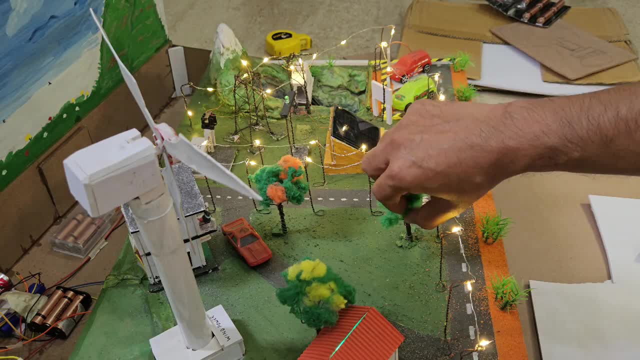 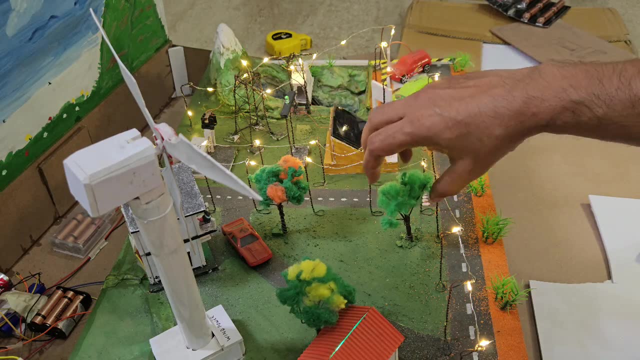 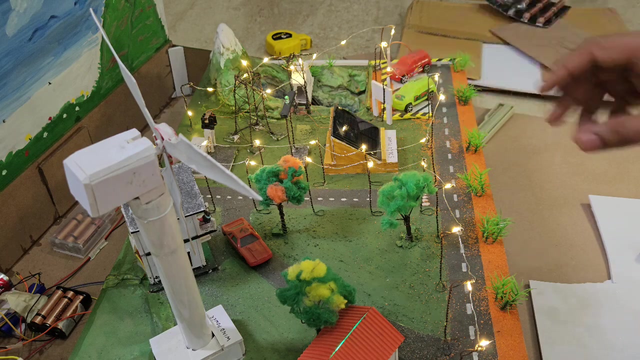 form like the canopy of this tree. so what's under it? i just cut the wires into various pieces. you can use any wire. you find rolls of wires or copper wires. basically these are the iron wires- very cheap to find in. basically these are used to when house is constructed, the wires they lock. 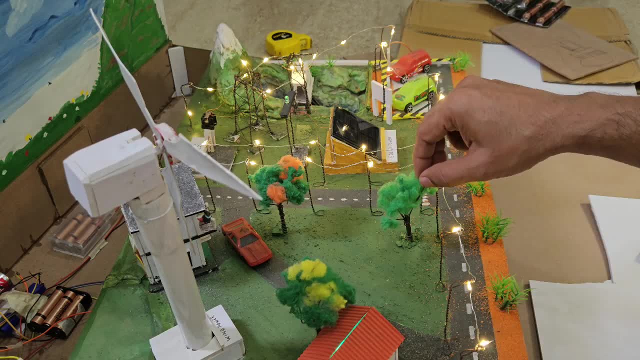 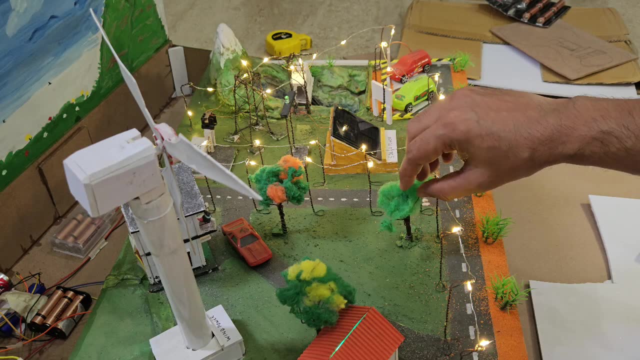 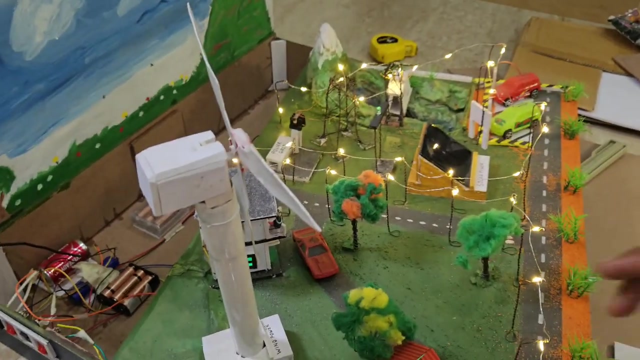 the iron bars with. this is that wire, so you'll find it easily. i cut it and bind them together to form on the branches of the tree and i just put it the colored cotton over it. so coming over to the next part of that was all about this windmill. now coming over to this next. 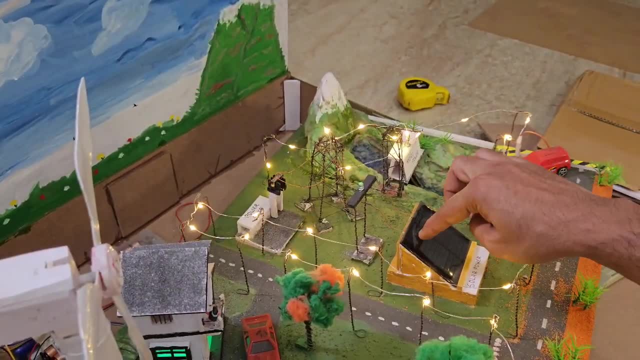 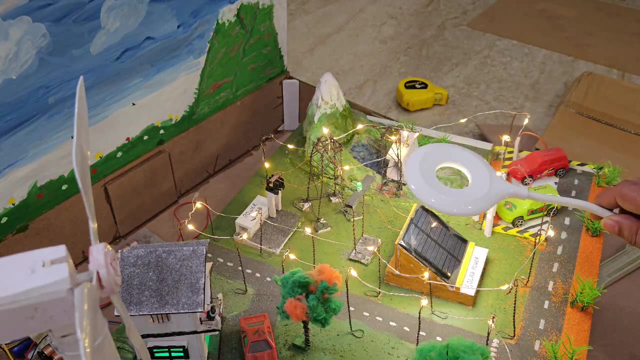 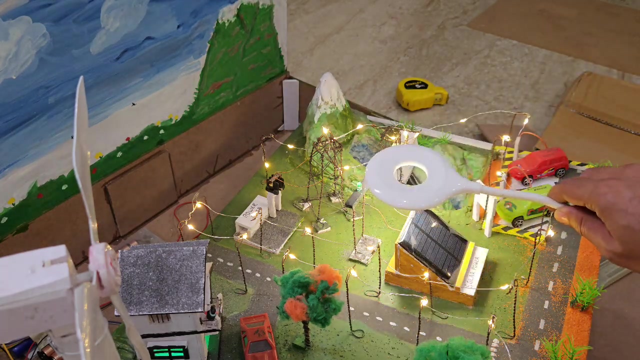 uh, this is very amazing: the solar power. so this is really actually working without the batteries. there is a bulb that is glowing. i'll just show you. it will glow a little more intense when i put the light over it. you can see that this is a bulb- led bulb- that's glowing with the power of this light. 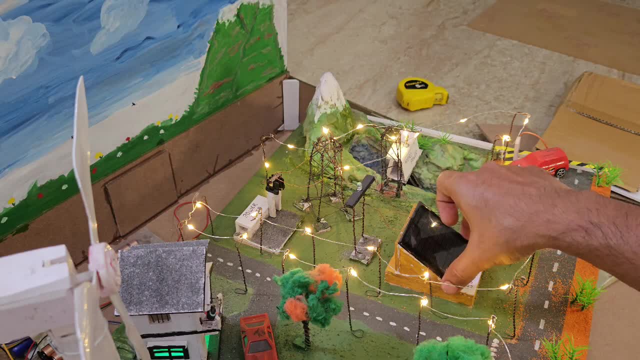 this is a solar power, so this solar panel, this is a single plate of a solar panel. this also you can find in amazon. you can just search it with the solar cell so you'll find this, this in thousand masterpiece. there is a wakees top that's going moment visiting this awesome. 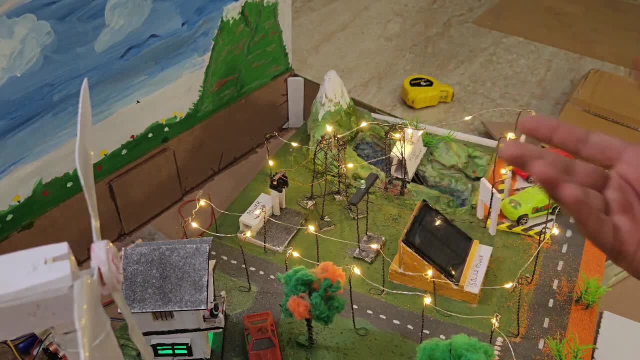 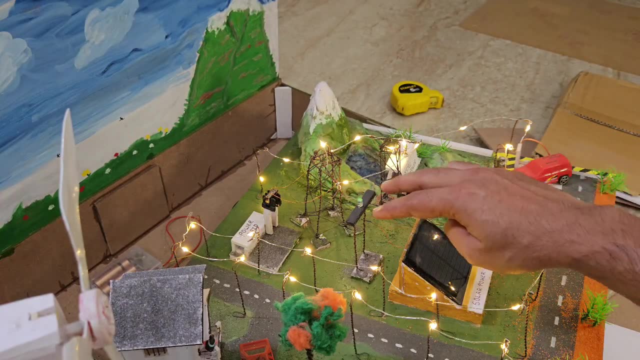 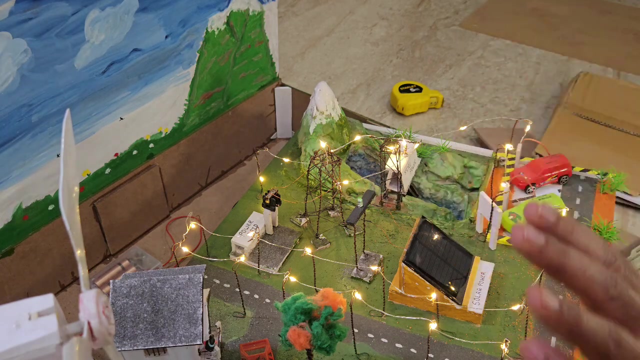 power tower is very powerful and you can see, i just made it with the same tool. um, i just made the base out of this soft. this is a foam sheet. i just cut it for the space, so i pasted over it, and the same glue- same glue from the glue- was used to paste this too. 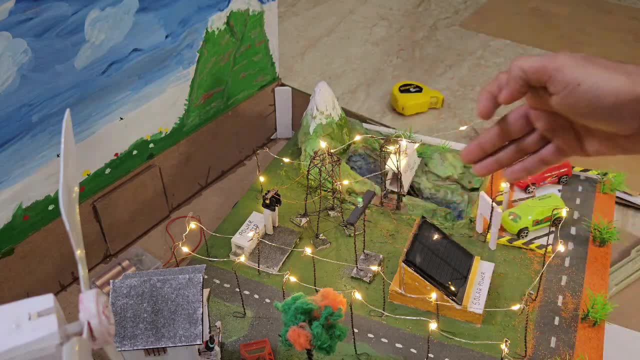 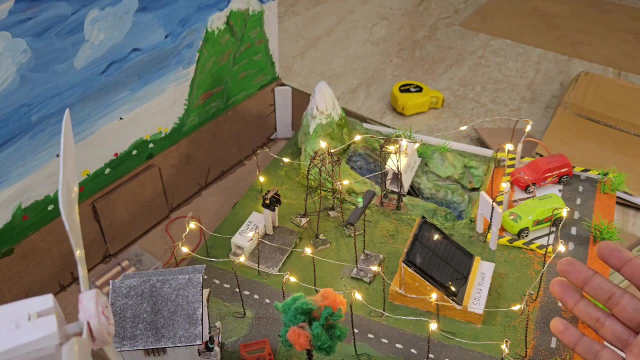 again was built with the same wire and i connected this whole led and can taken it down to the battery pack that was provided with this led. so these are the wonderful thing about this led: that you can cut it to any length of your requirement. so next is the hydro power. it was quite challenging to 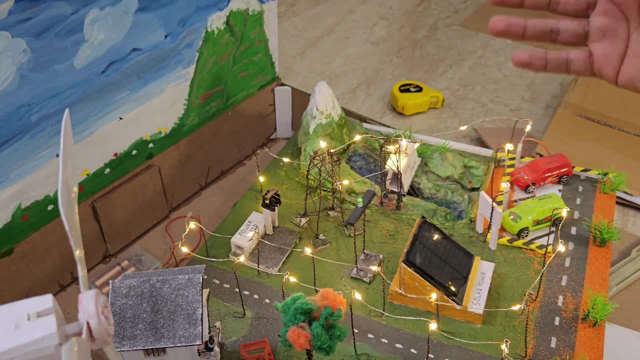 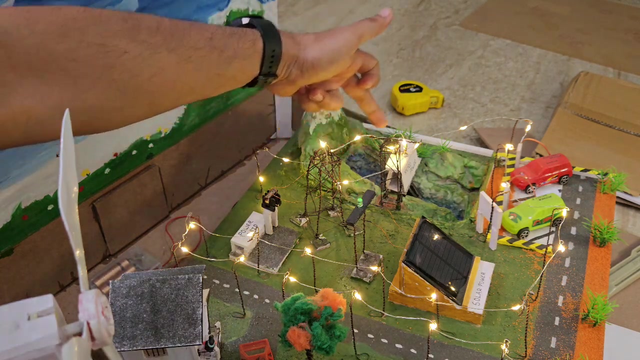 build. a thought process was, went to it many a times. i just wanted to create the realistic, so i created it. what exactly? how it's working. it's quite interesting. so what i tell you? it's exactly. the water flows here from this part and goes down again into a box, so under it there is a plastic. 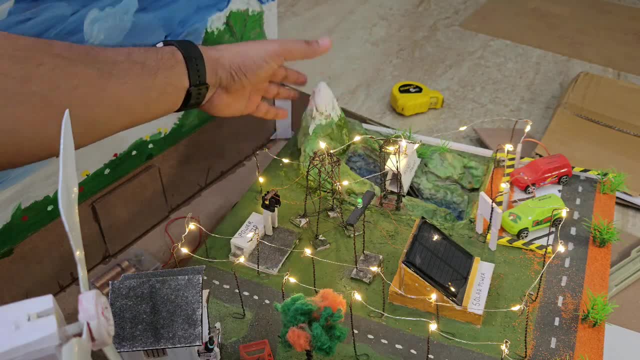 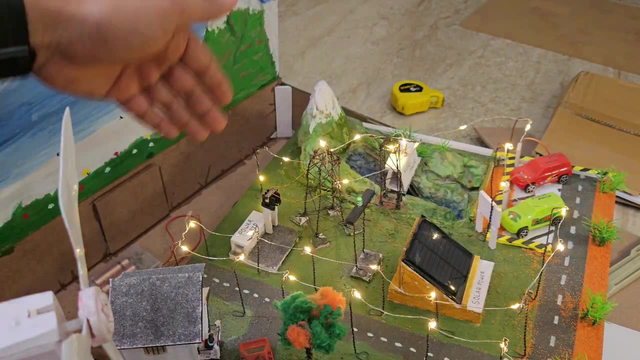 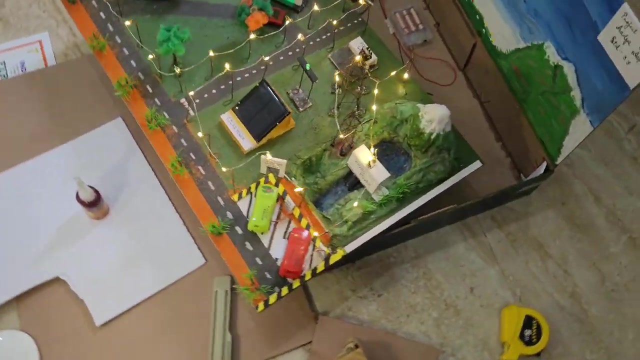 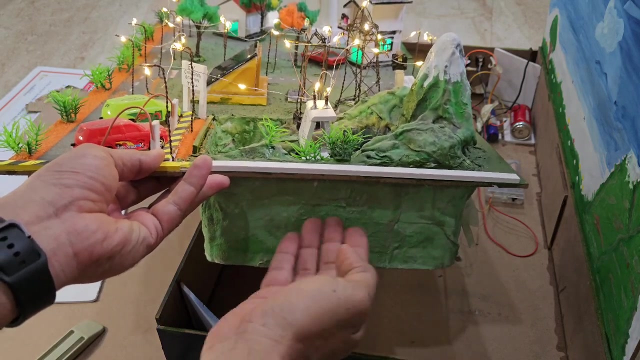 box that you can find in your home, that you keep. basically, it's a bread box of this same size, same length, from here to here. it's fitted under this, under this part. that was made this box. so i'll just show you how it's fitted. so here it is. you will have an idea how this box was fitted. so this is the whole box it contains. 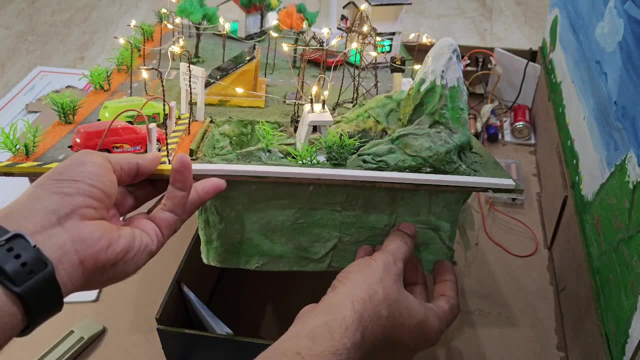 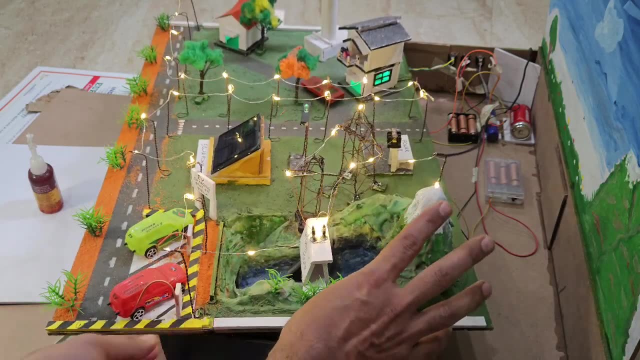 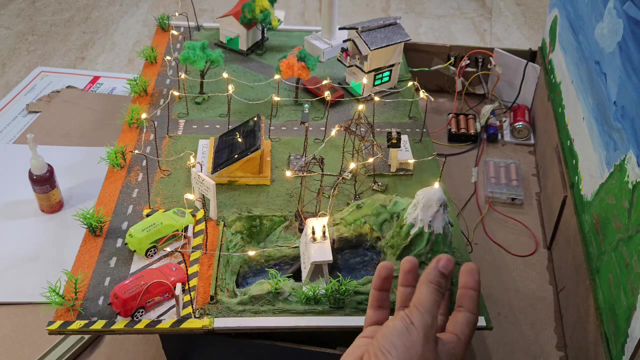 a water pump, again from amazon, and the pipe was connected under here and this whole mountain. it's exactly built with the cement, the cement that you found easily at home. i used the cement and to raise this, i used these thermocol foams to give it a shape and put it over. 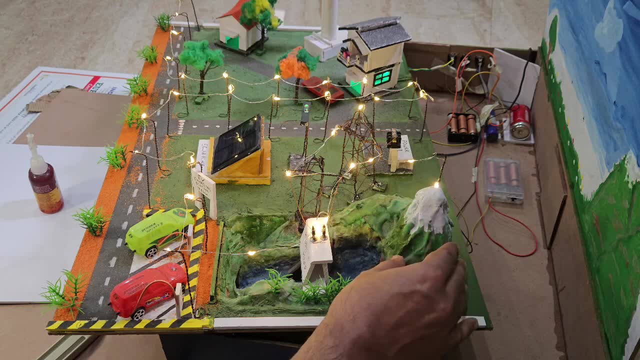 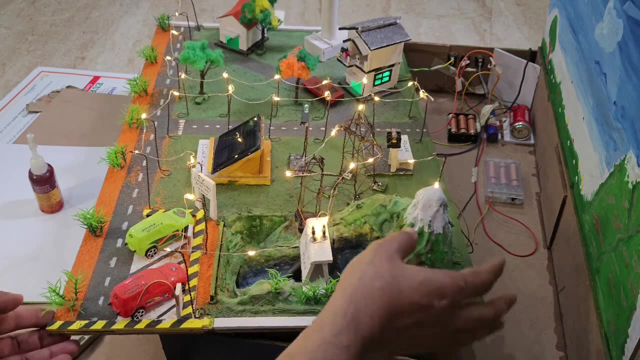 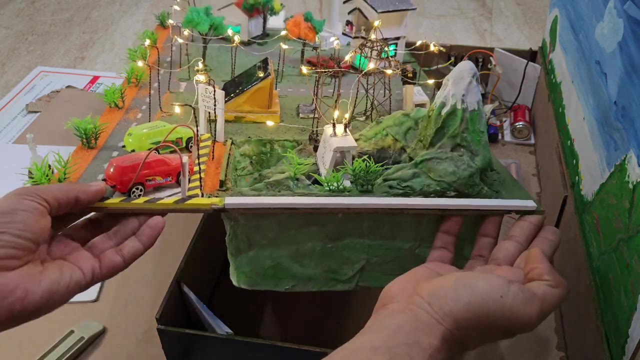 some cement and let it dry, and this would hold a shape of a mountain. and then i painted with the acrylic paint, so it was built in such a way that it hides all of the part, and then a hole was cut through over this upper sheet that you see, and just i fixed it under it and pasted it. 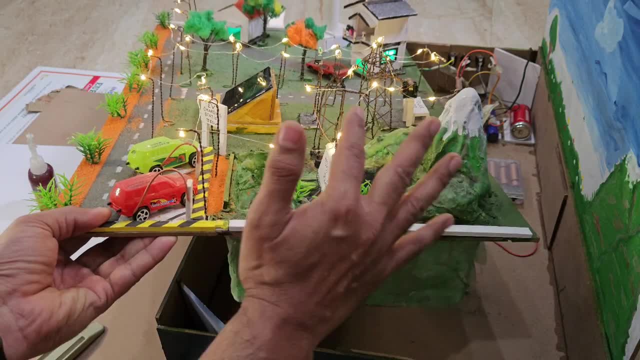 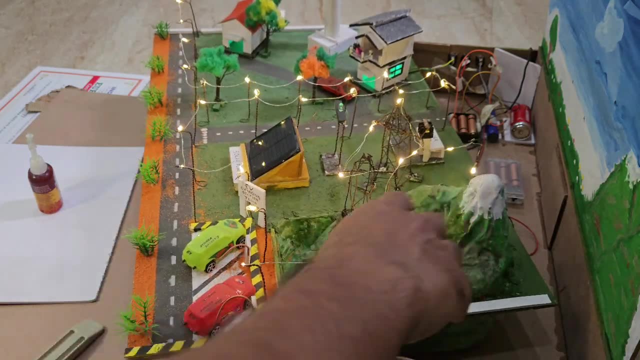 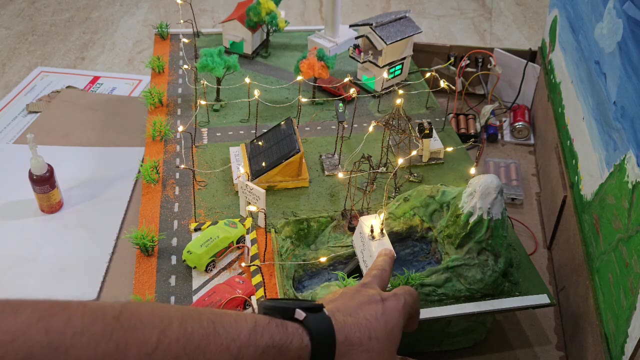 again so it not let the water to flow anywhere else. the fort with the water rotates inside this hydro, so it mimics the water flow of the mountain to generate electricity through the power of hydropower. so basically, the power, as you see, is separate for each of. 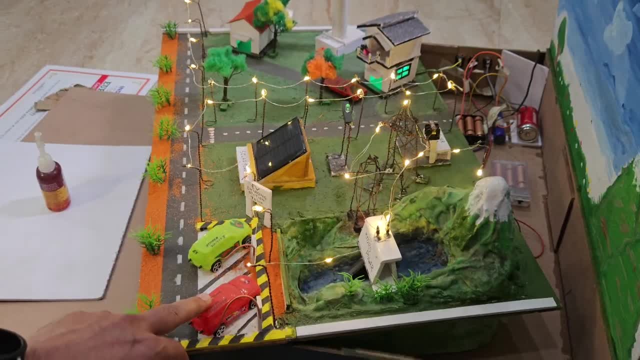 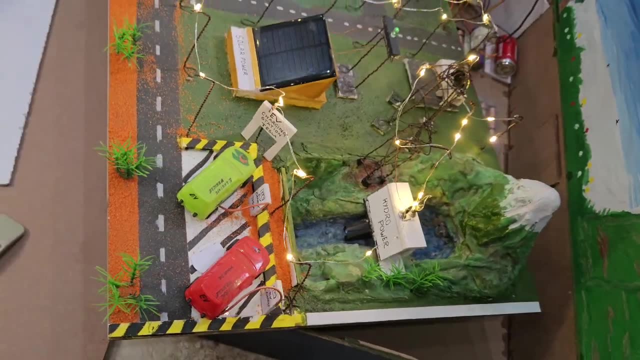 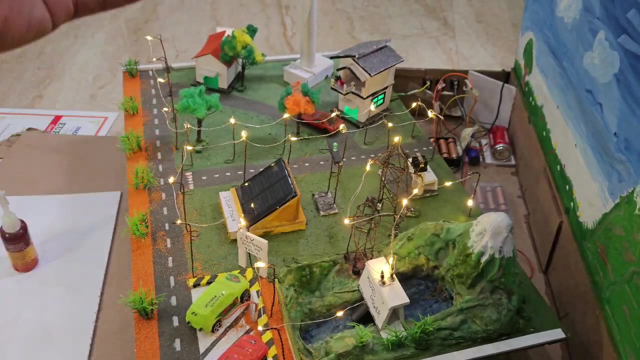 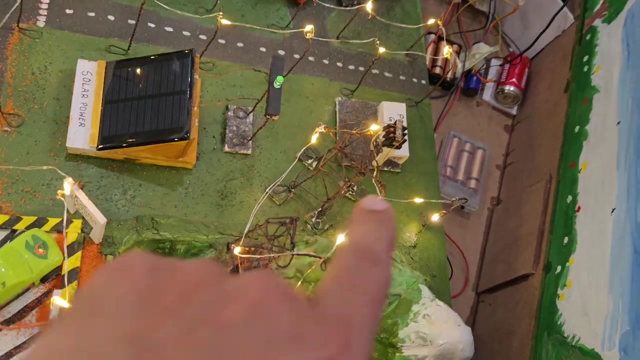 the project. so these cars were the toy cars. I built an EV station, EV charging station- again, model of renewable energy and how it can be used in various forms. it depicts the forms of various forms of energy and again we have a power grid station. you see a small little transformer over here. it's an power grid. 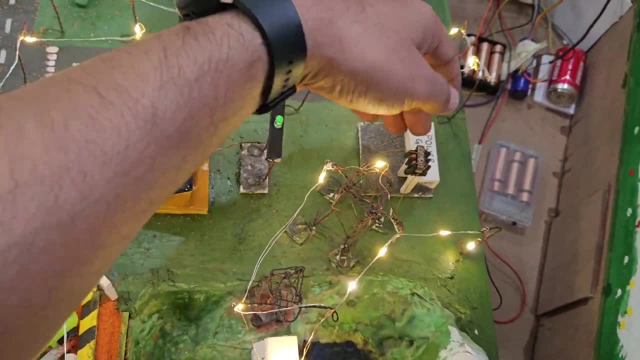 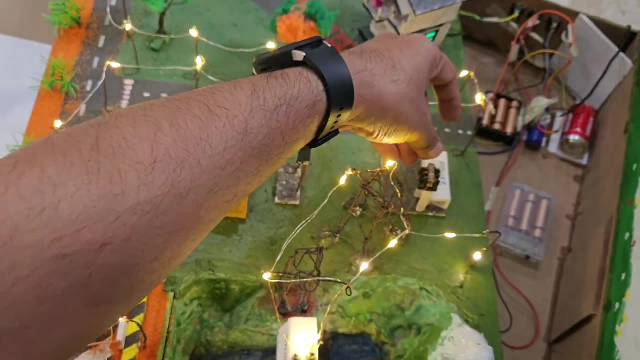 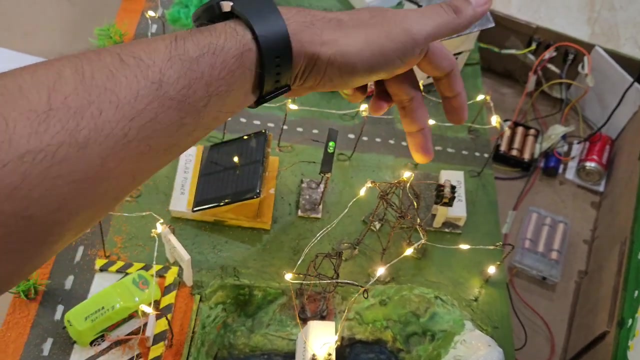 mimics, power grid, so how it was built. this transformer are found in the old charger line, your mobile charger, anything, any kind of chargers or anything. you can find this small transformers inside them. so it's in just a depiction of an transformer. how the power, the power. 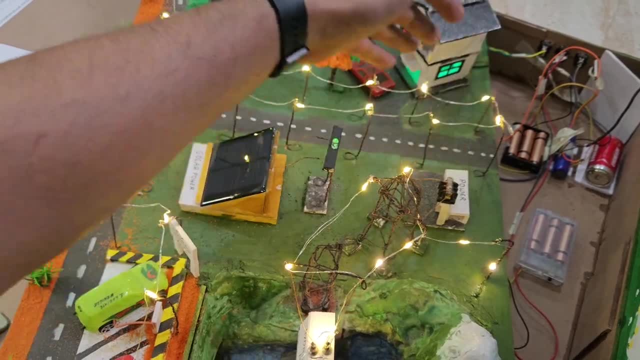 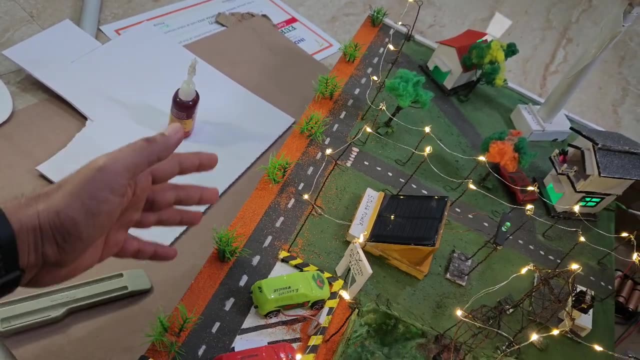 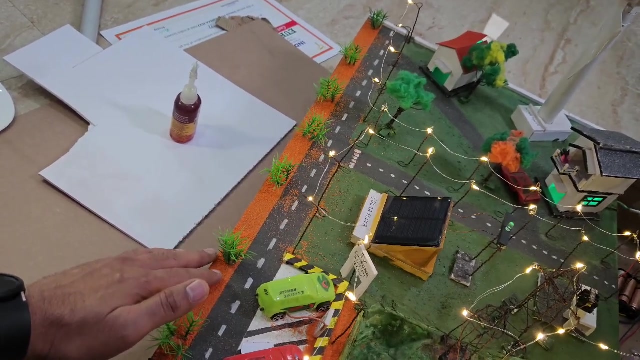 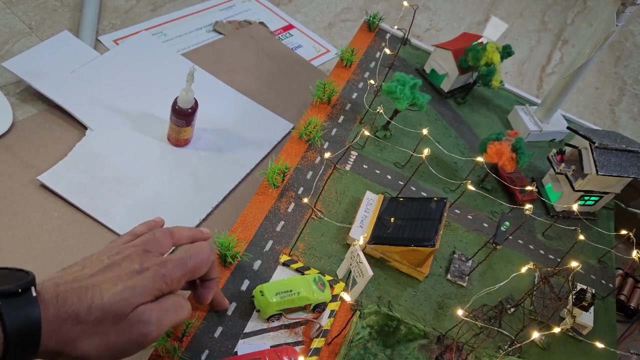 lines, electricity it generated any step down to a domestic use. so these are some of the mass pieces that was again from Amazon. you can order it. and these color sand that was bought from them stationary store you can find. and these roads, these are painted with the acrylic paint, black acrylic paint marked. 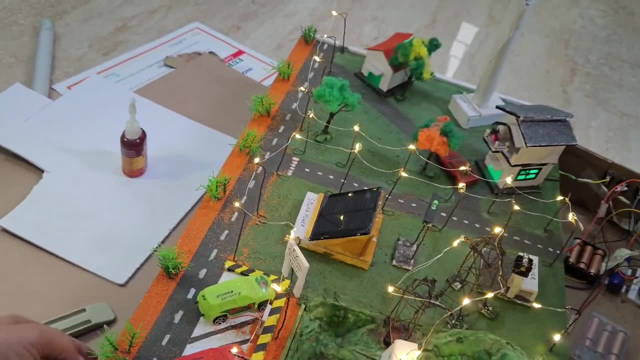 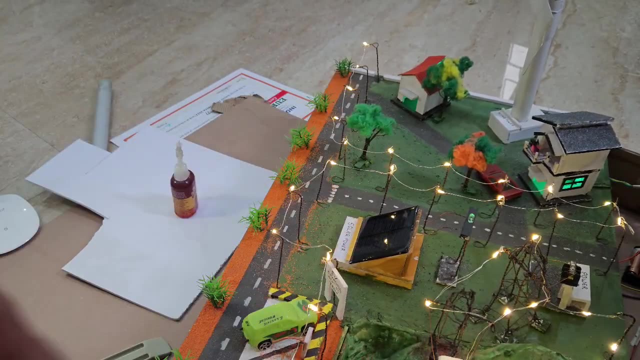 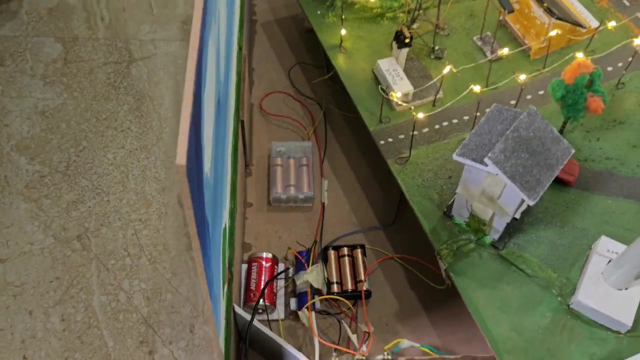 the white acrylic paint and this whole area, you see, is the hard board and over it we have just painted color with the green. so let's coming over to the connections, electrical connections that are placed under the box so they're hidden away from the box. the first one you see here: it provides the electricity. 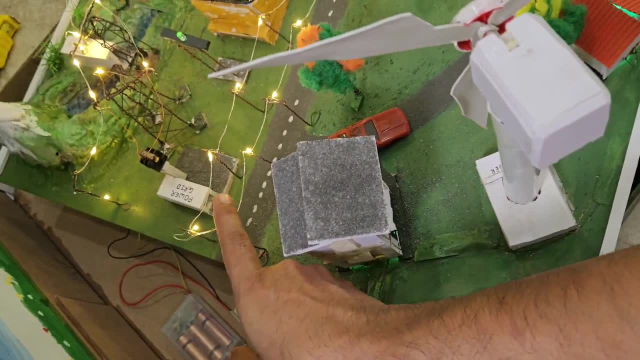 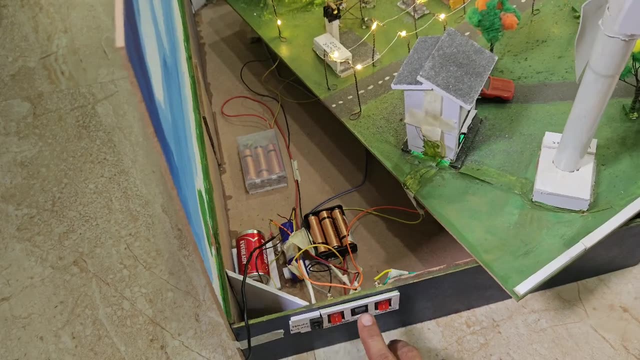 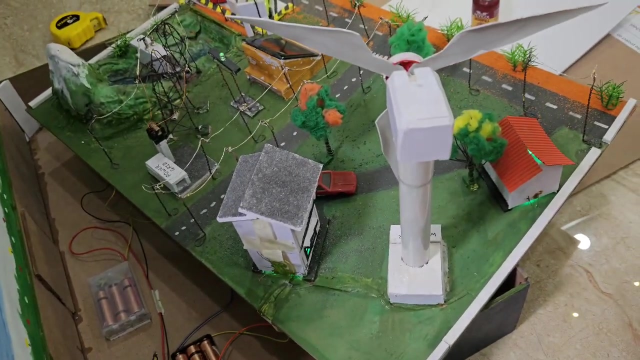 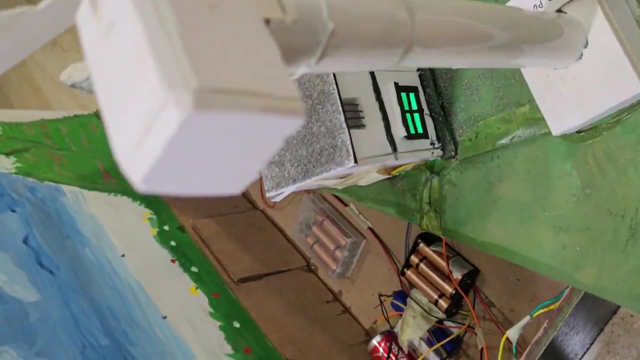 for these street lights that we have put. okay, so here we go, and this was connected to a switch that you can see over here so you can turn it on and turn it on and turn it off, according to your convenience. the next one, the next switch: we have connected to the lights for the houses. 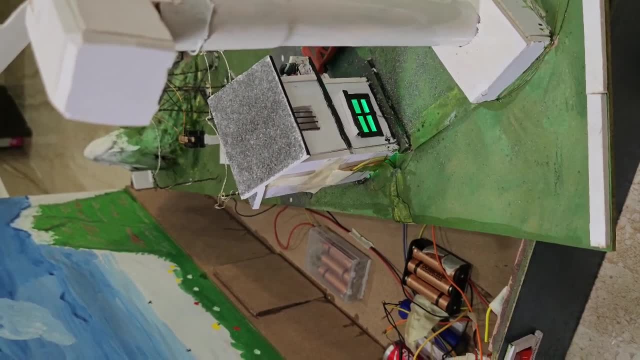 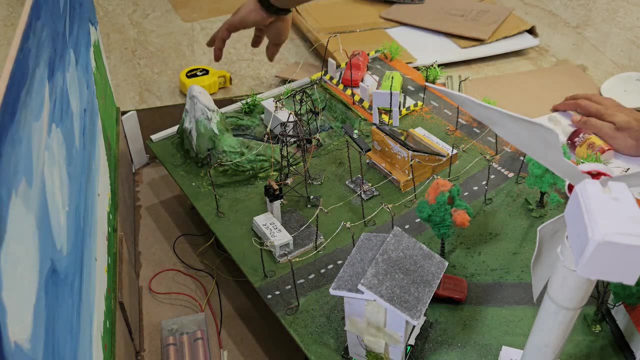 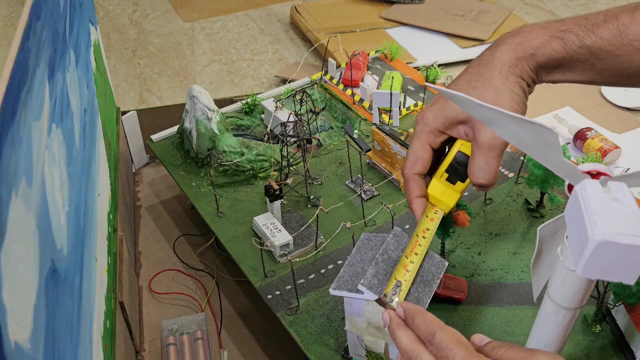 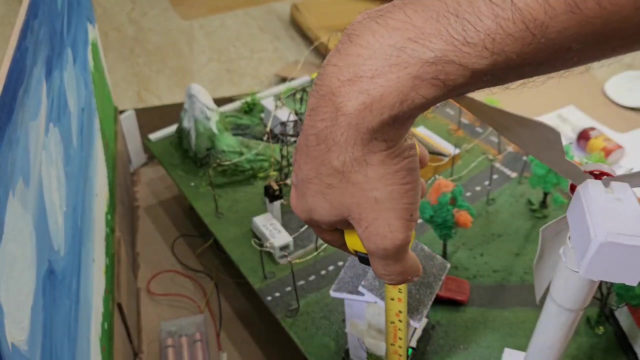 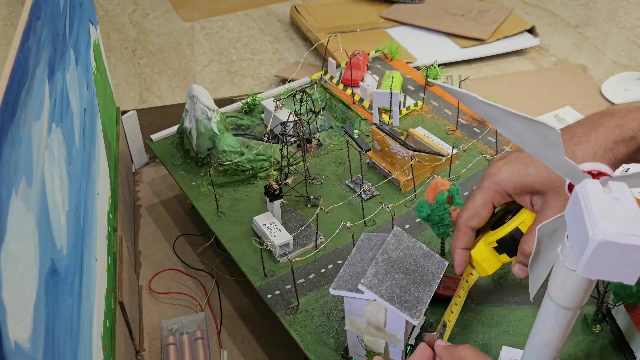 you can see. so let's again. so again, I'm going to measure it for you. the roof is around three inches wide and the total house height is around four inches- a measurement that you can build easily- and six centimeters in the width. it's around six centimeters. the roof for the another house was built of a 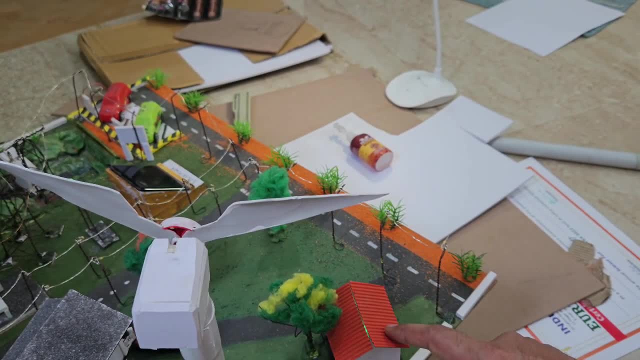 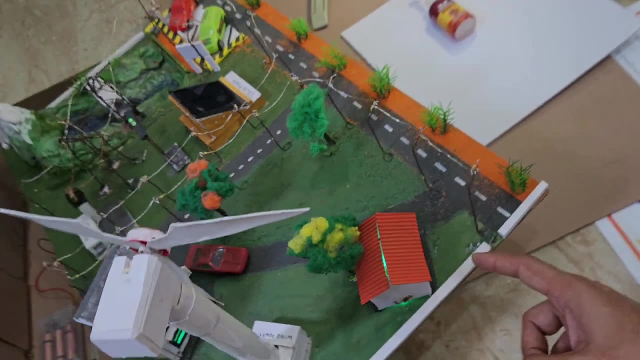 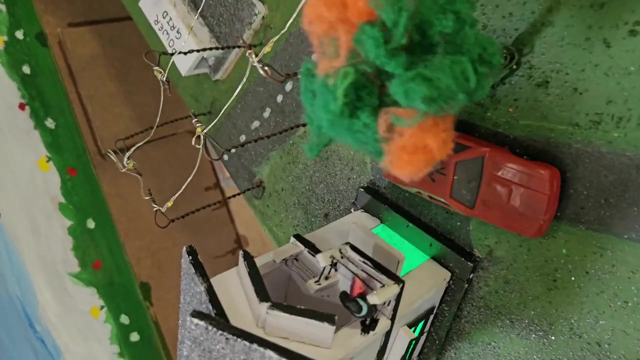 cardboard that you easily find, and it was painted with an acrylic paint again. the LED bulbs are connected under this, so the light is just coming through. I'll just show you. so the house has the cards and the house has the lights. so this was all about this house. 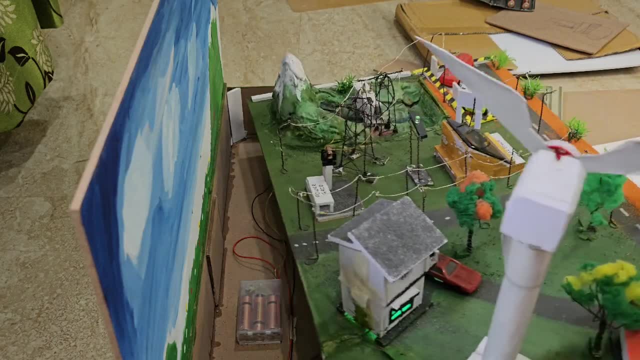 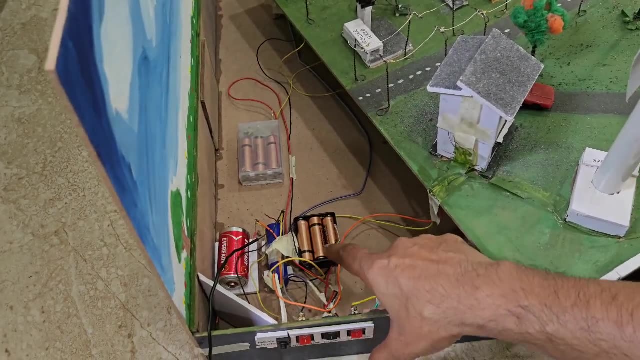 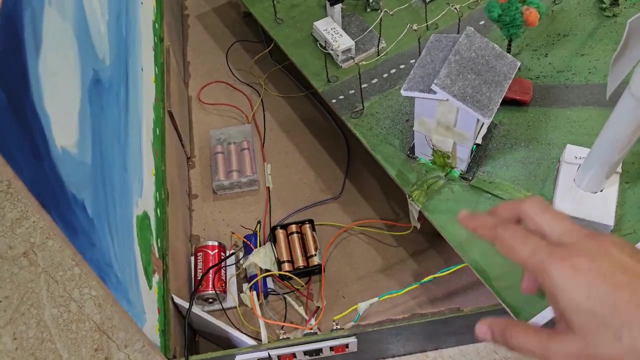